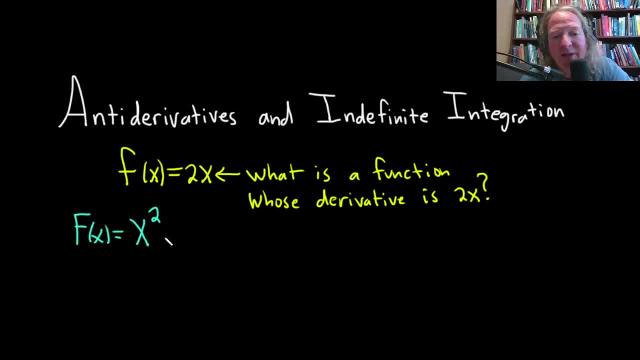 I'm going to call it big f of x, And this is an example of what's called an antiderivative. So this is an antiderivative. So we would say that x squared is an antiderivative for 2x. 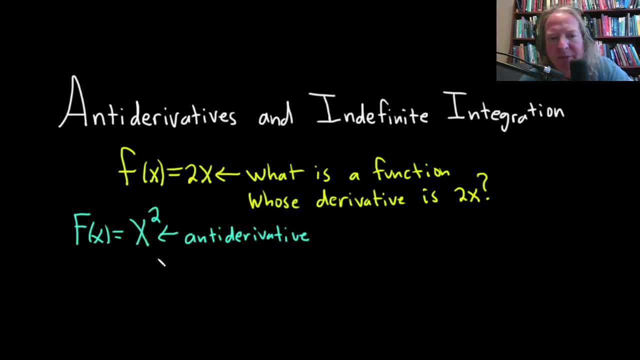 because the derivative of x squared is equal to 2x. So the thing is, there's other possible answers. For example, let's say I say big f of x is equal to x squared plus 1.. Well, if you take the derivative here, you're going to get the same thing. You're going to get. 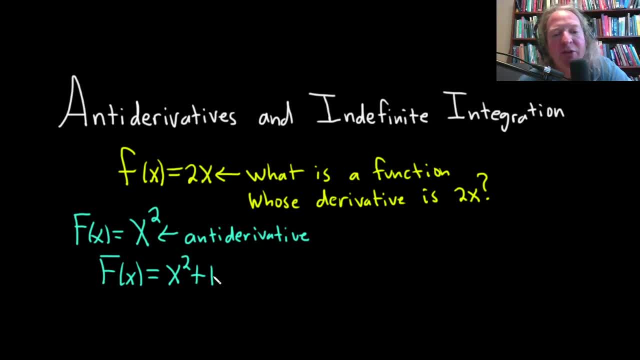 2x. The derivative of x squared is 2x and the derivative of 1 is 0. So you're going to get the same answer, But this is also an antiderivative for 2x. In fact we can look at big f of x. 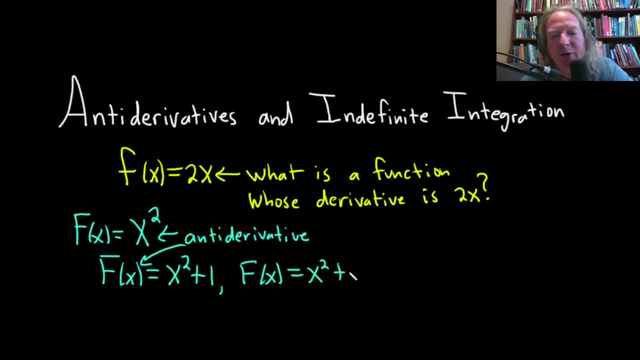 and call it x squared plus any number, I'll use a capital C, And this is also an antiderivative for 2x. This one has a name, This one's called the general antiderivative And this C here it's an arbitrary constant. That's the word we often use. 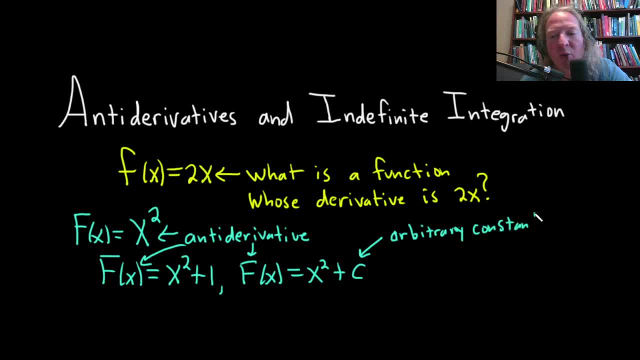 Arbitrary constant. So it could be any number. We don't know That's an R there- Arbitrary- This is hard to read, So A-R-B-I-T-R-A-R-Y Arbitrary constant. So there's infinitely many. 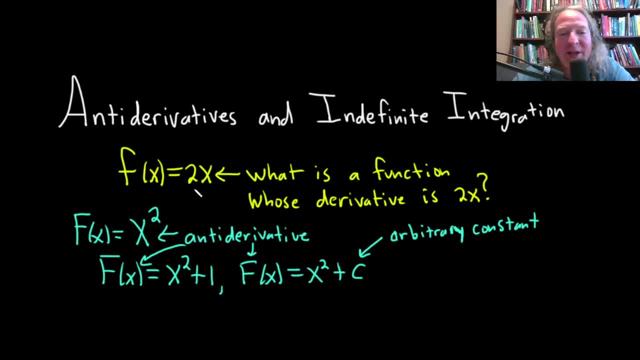 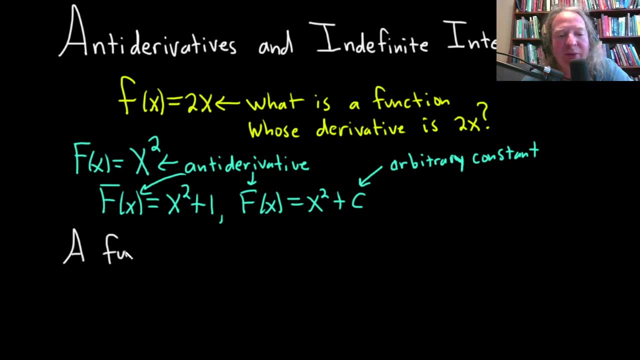 antiderivatives for 2x. Let me just go ahead and give you the definition, so you have it in some place. So we say a function, big F is an antiderivative, So antiderivative of little f on some interval i. So I'll say on an interval i. 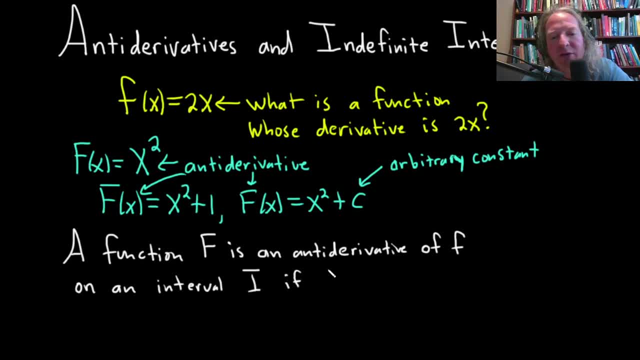 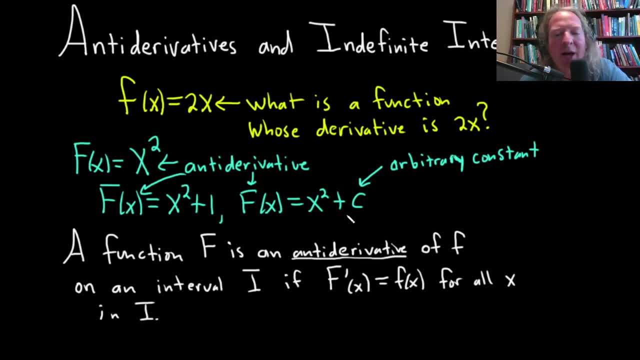 of an antiderivative, And typically in a calculus class you do use this, But in the actual problems that you do in calculus you don't use it too much. So it would come up a little bit more in maybe like a proof-based class or something like that. The point is though: 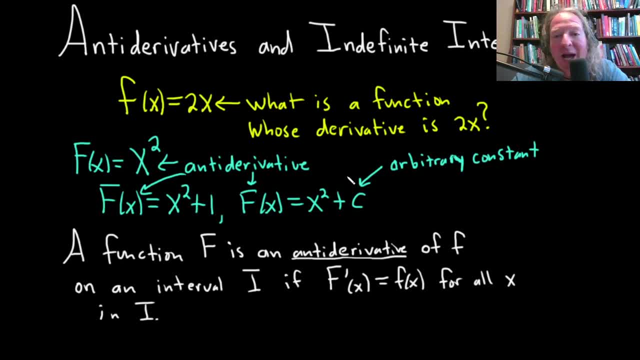 that there's infinitely many antiderivatives for 2x. So this is an antiderivative. many, right, there's infinitely many. and now let's talk about what integration is, and I'm going to give you the notation. I'm going to switch colors here. oh, 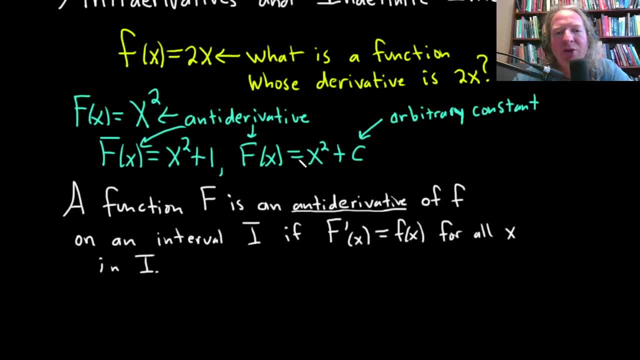 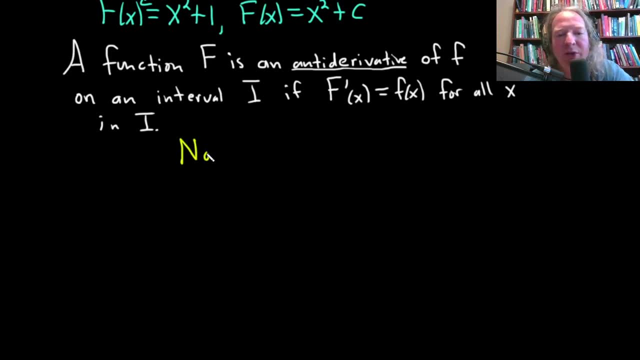 before I do, though, let's actually do it with respect to this example, so that way doesn't look so abstract. so here's the notation that we're going to use. so the process of finding an anti-derivative is called anti differentiation. right, we're going backwards. so instead of differentiating, 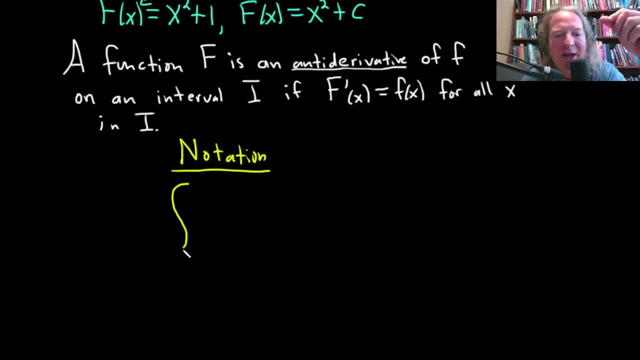 we're anti differentiating and here's the notation we use. so we have this elongated s symbol. this is called like the integral symbol, so it's the integral symbol. and here we have 2x and then we have DX, and we said that our best answer was this: one x squared plus C. 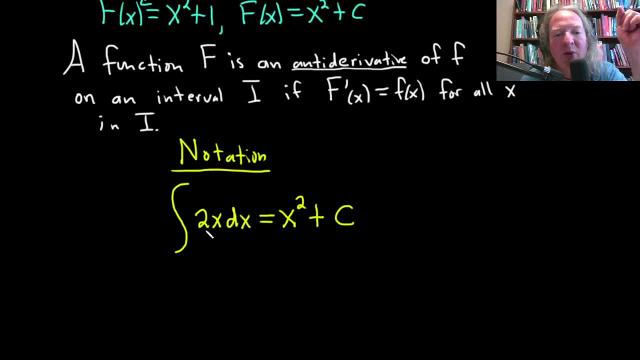 this example which we did in our head. we looked at the 2x and we said: what? What's a function whose derivative is 2x? We said x, squared. This is the notation you would use. So this process of finding an antiderivative is called anti-differentiation or integration. 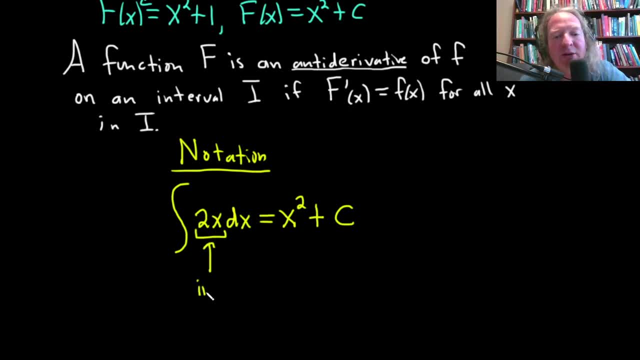 So this piece here has a name. This is called the integrand. It's really important to know this, because when you're talking to people about mathematics you say, well, my integrand, you know I couldn't factor it or you know you can talk about. 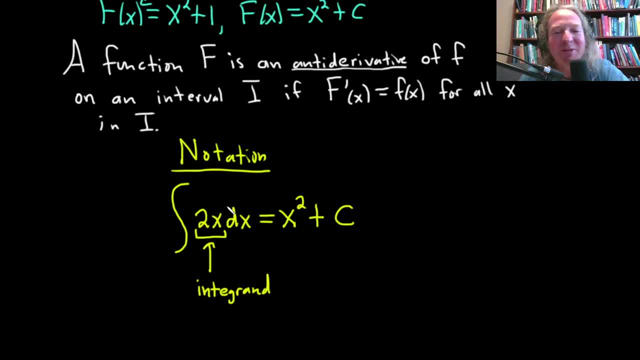 the integrand, because you know what it is. This piece here, this dx, this tells you what variable you're integrating with respect to. So I'll just say variable of integration. So, because it's math, we have more than one variable. 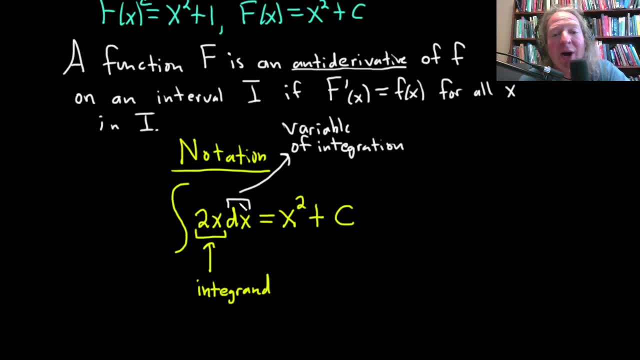 Sometimes we integrate with respect to y, in which case you would put a dy, Sometimes you do theta, Sometimes you do r. If you study multivariable calculus, you'll do x, y and z in the same problem, So you'll have dx, dy, dz, dx. 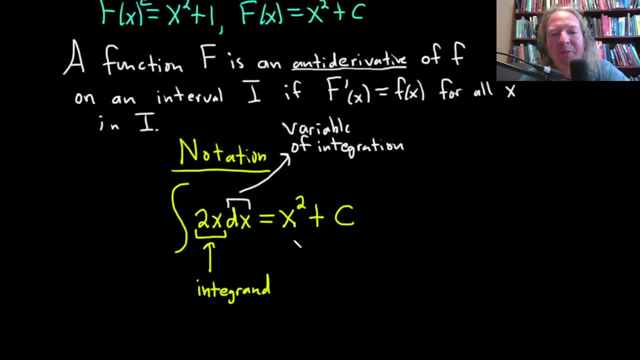 So it tells you the variable. So here the variable is x. This here is our antiderivative: x squared. In fact, this whole thing is an antiderivative. You could say x squared plus c is the antiderivative, but I'm just going to single out x squared. 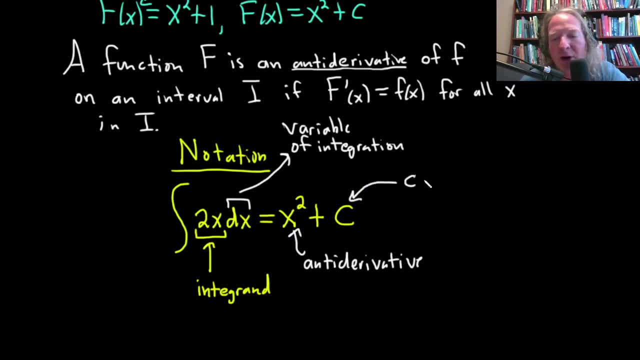 just so I can label this one as well. This one has a name. We called it an arbitrary constant, but it's actually called the constant of integration. Okay, That's it, That's it, That's it. It's the constant of integration. 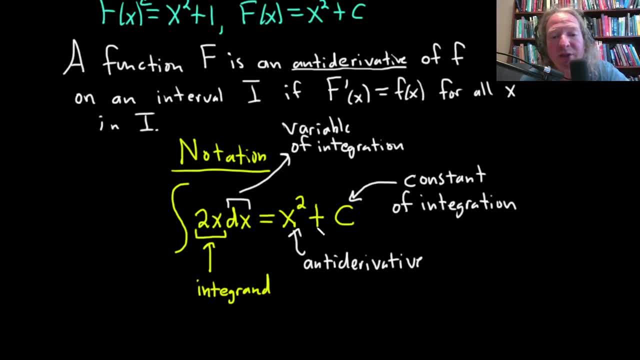 It's really important to include it. There's infinitely many solutions right. There's infinitely many choices for c. There's infinitely many antiderivatives- really, really important to note. And this elongated s looks like someone took the letter s and stretched it. 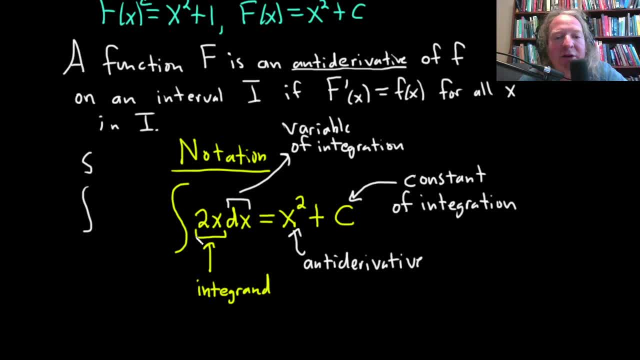 This is the integral symbol. So again, this process of finding a function whose derivative is 2x, this process of going backwards, it's called anti-differentiation or integration. Okay, This is called an indefinite integral. So indefinite integral. 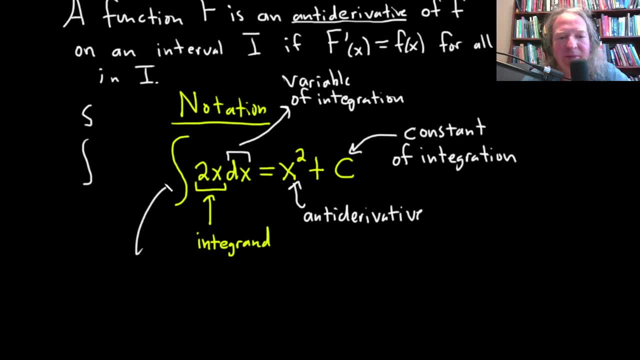 I'm going to write that down. So this is an indefinite integral. A natural question then comes into play: What is a definite integral? A definite integral is different. You're going to have numbers here. You might have a 3 here and a 4 here. 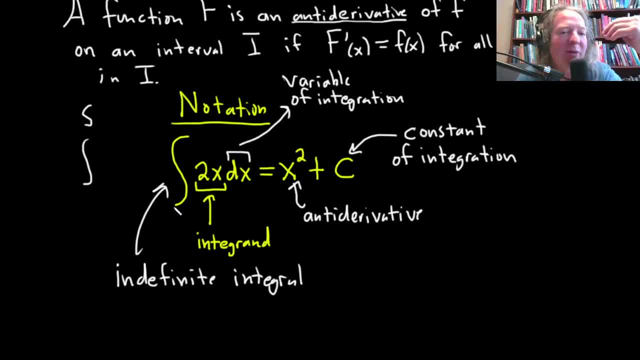 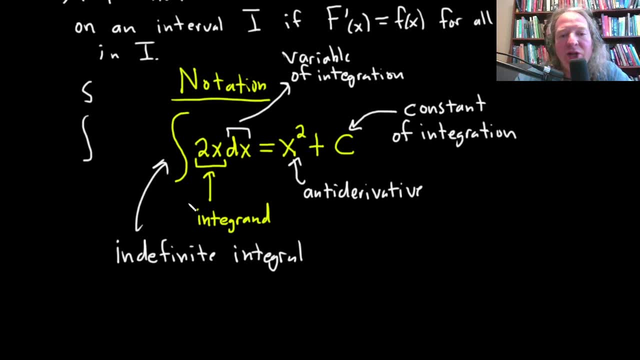 That's called a definite integral. Those are studied later. You have to learn about Riemann sums and some stuff like that, But for now we're going to stick with indefinite. So in general, to do this it's pretty tough, right. 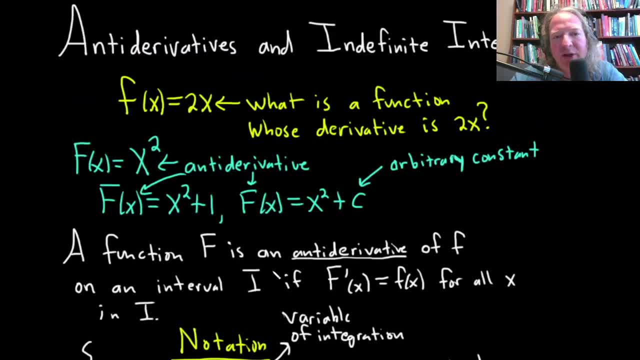 Like we had to. you know, I picked this example for this video because it's easy, right? So I wanted to pick something that most people who know very, very basic calculus can do and understand. Yeah, okay, what's a function whose derivative is 2x squared? 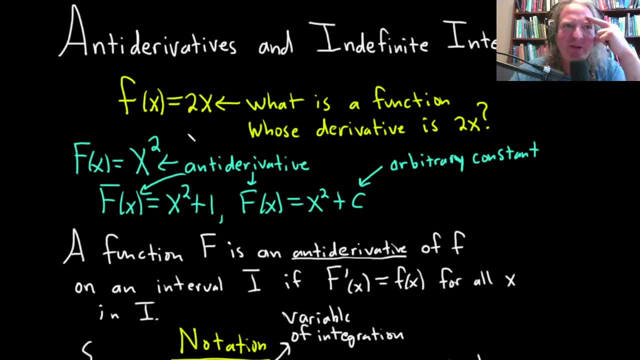 But if I say, hey, what's a function whose derivative is, you know, x plus 1 over x cubed plus 1 minus the secant of x, Like you know what's that going to be? Well, it's a little bit more difficult, right? 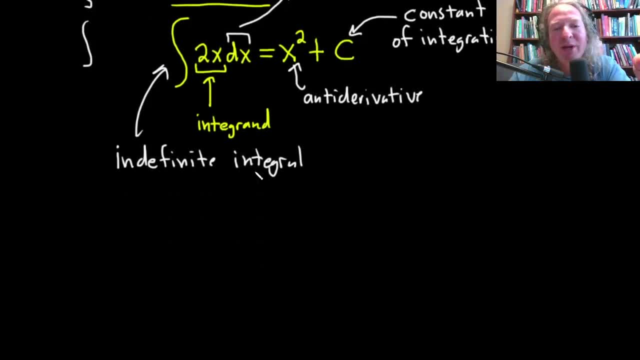 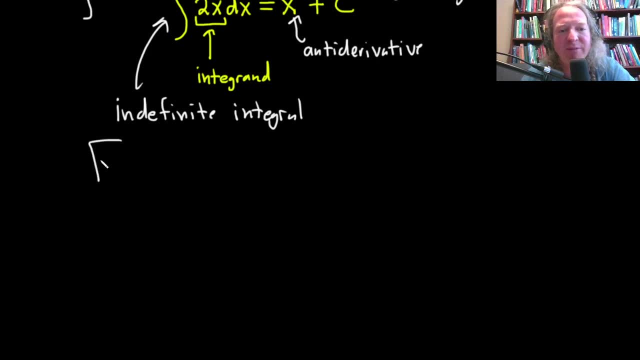 So you need formulas in order to do these problems. So now I'm going to give you a list of all of the basic formulas that you need for integration. So formulas, And we'll justify each one at least logically, And in some cases I'll be able to give you an example. 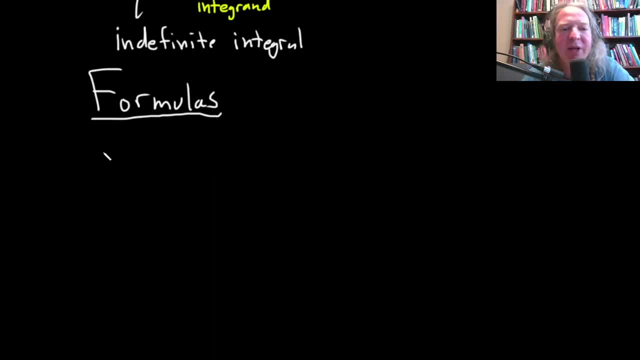 In some cases I really won't, not until later. So the first formula we're going to look at is, if we're trying to integrate 0,, okay, 0.. We're looking for the antiderivative of 0.. We're trying to anti-differentiate 0.. 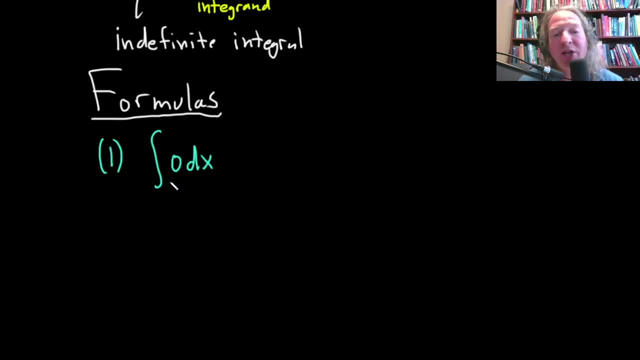 So lots of ways to say similar things. So this integral, we have to integrate 0.. So you ask: what's a function whose derivative is 0?? Well, any constant function. We'll work. Let's just go with c, right. 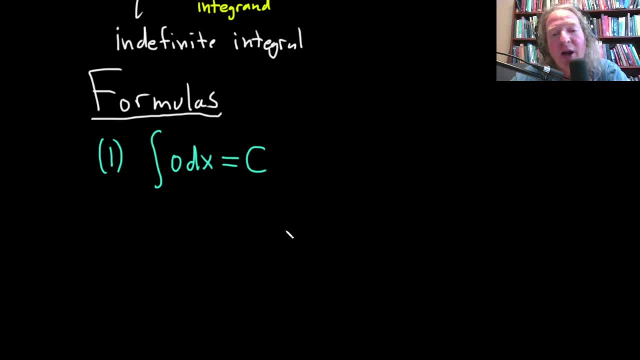 c will work, Because if you take the derivative of c, you're going to get 0, right, The derivative of a constant is 0. So that one's pretty easy. How about this one? Let's say we have a constant which I'll call k. with respect to x. 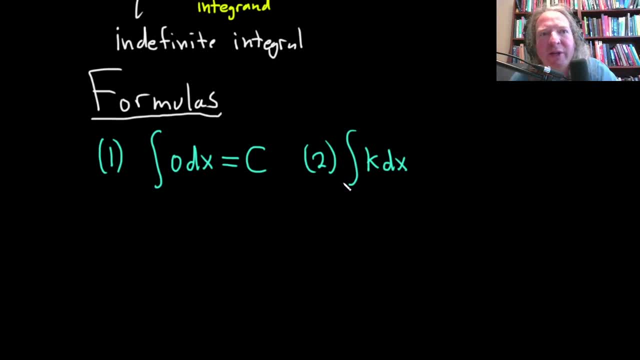 So the variable is x. What's a function whose derivative is x? Well, it's going to be kx. And then, of course, plus our constant of integration, And you can always Check your answer. If you differentiate this, you should get the integrand. 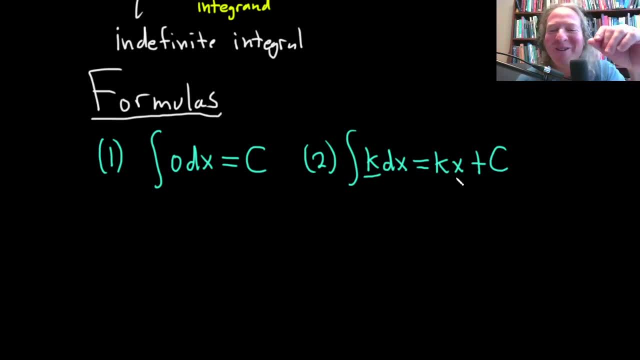 See how important it was to know what it's called. It helps to know. So the derivative of x is 1.. So we just get k And the derivative of c is 0. So it goes away. Let's do an example with this one. 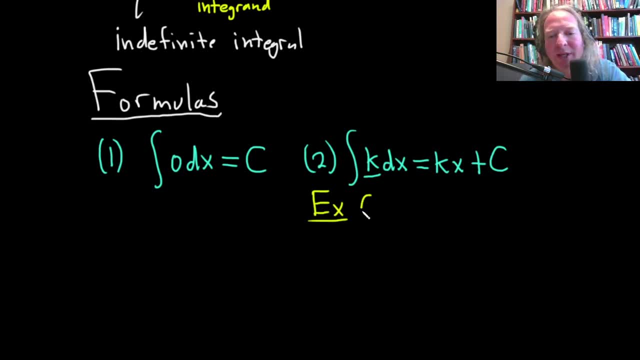 We can do a simple one. Let's say we want to integrate 2 with respect to x. So in this case there's two ways to do it: Method 1. You ask yourself: what's a function whose derivative is 2?? 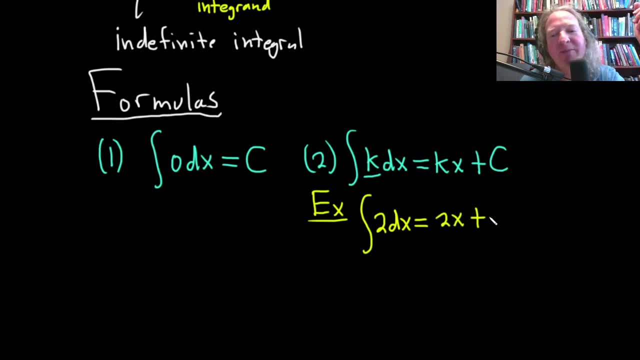 Hmm, 2x. And then don't forget the plus c, Method 2, which is the way I do it, which is much more mindless. It requires less brain cells. You see the 2. It's a constant by itself. 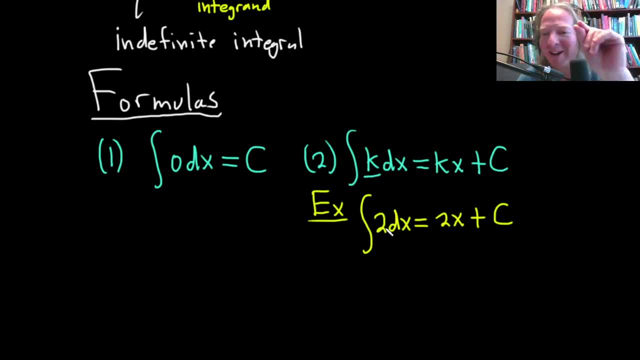 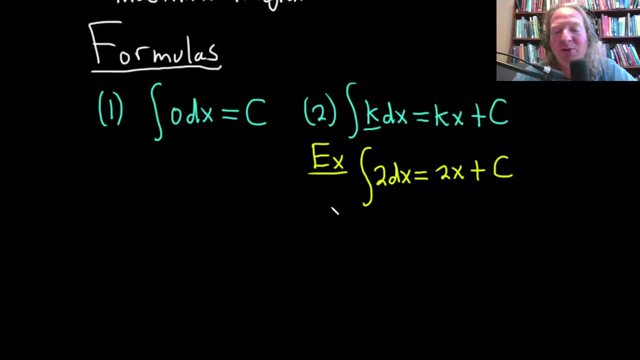 You just put an x next to it. Simple right. Doesn't matter how tired you are or how much math you've been doing. If it's a number by itself and it's with respect to x, you put an x. Actually. this leads me to a point. 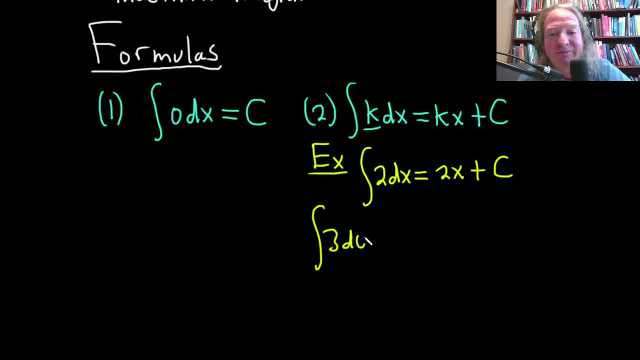 Let's say instead it was 3x. Let's say instead it was 3d theta. What? What's going on, Trig? Yeah, I want to introduce a theta. Why not? Right? So in this case it's 3 theta plus c. 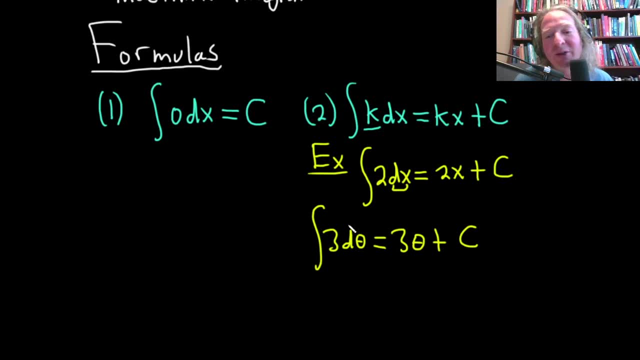 So it depends on the variable. That's the purpose of this. It tells you what the variable of integration is. So in this case it's d? theta, So we put a theta. If it's dr, you put an r, etc. 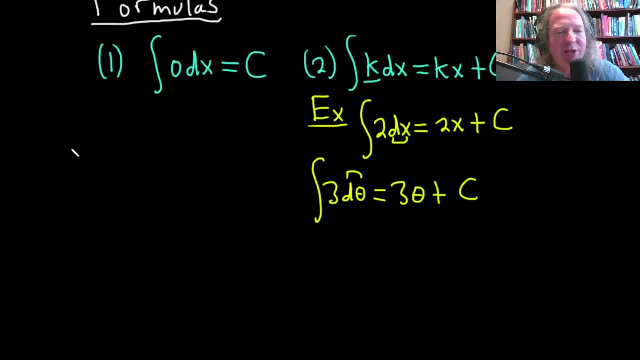 All right, Let's go to our next formula, which I'm just doing these off the top of my head. How about this one? If you have a constant, If you have a constant times a function, you can pull the constant out because it doesn't. 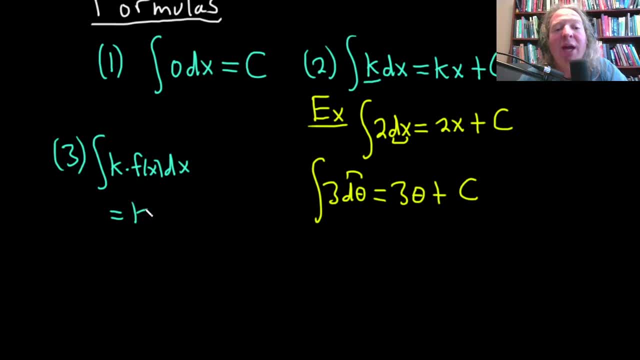 depend on the variable x. So this is equal to k times f of x dx. This will come up sometimes later. Just know that if you have a number you can pull it out and there's no issue. As a concrete example, I guess I could do one here. 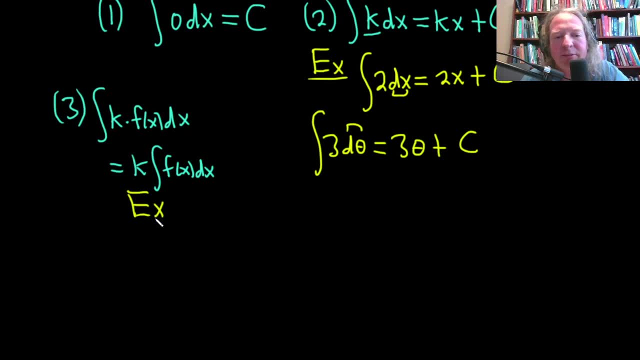 It's a little bit silly, but let's do it. Let's say you're trying to integrate 5.. With respect to x, you're saying: huh, I don't really like the 5, so I'm going to pull it out. 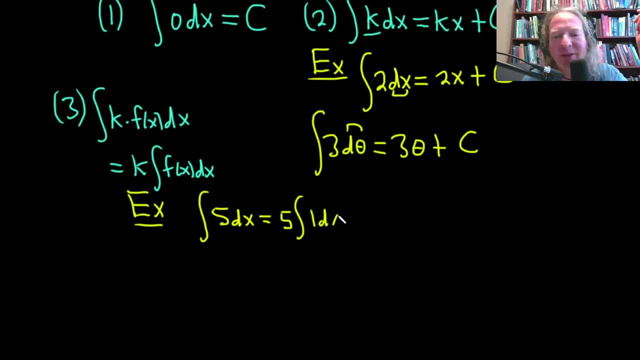 So you pull it out and you're just left with 1 dx and you say, oh, 1, I can integrate 1.. That's just x, Right, Because 1 times x is x. The derivative of x is 1.. 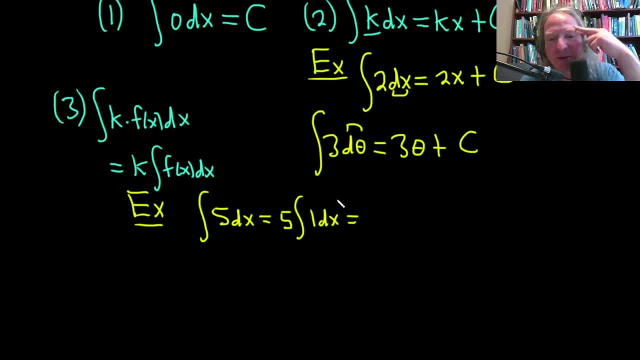 So the integral of x, integral of 1, is x rather. So to integrate 1, you just use this rule right. So you just put an x next to it, but you just get 5x. Let's see So a pretty useless move here. 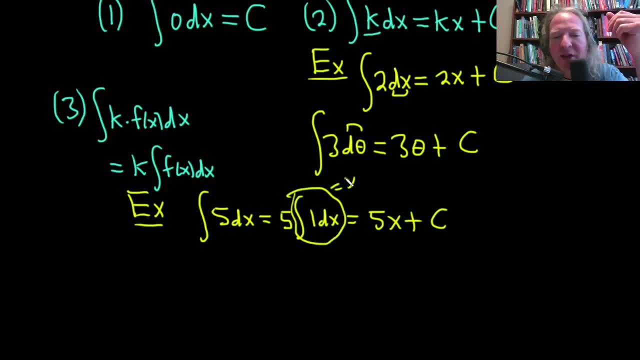 Right, So you integrate this and you get x, and then you just multiply by 5 and you get your answer. So not very useful in this particular case, kind of a pointless example. But the point is you can pull numbers out which can be useful sometimes, just not in. 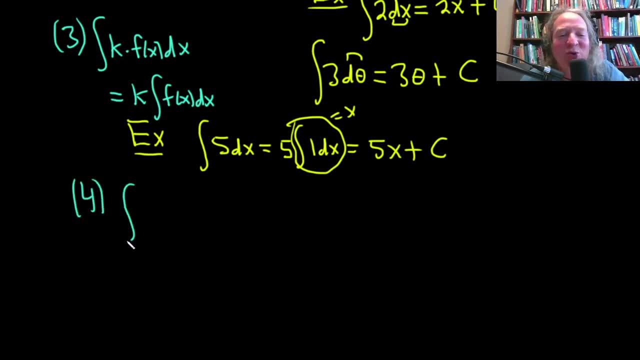 this particular case. here This next rule is very useful. It says: if you have more than one term in your integrand you can separate it into two integrals. So if you have, say, f of x plus or minus g of x, 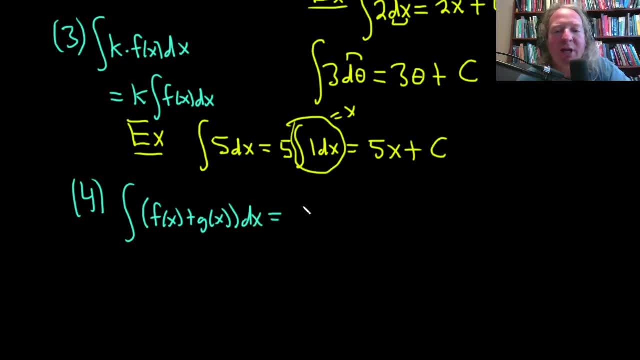 Right With respect to x. You can break this up into two separate integrals. We have the integral of f of x with respect to x, plus or minus the integral of g of x with respect to x. Very useful, And once we know more, I can do an example of this. 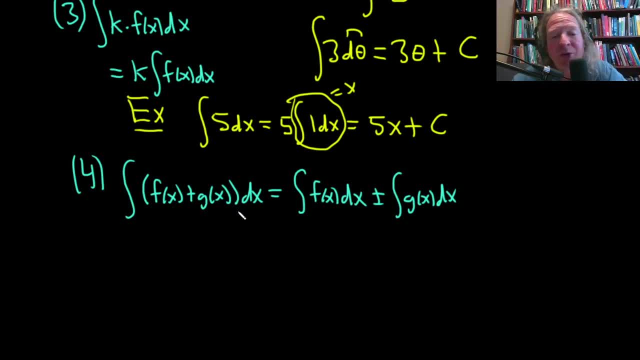 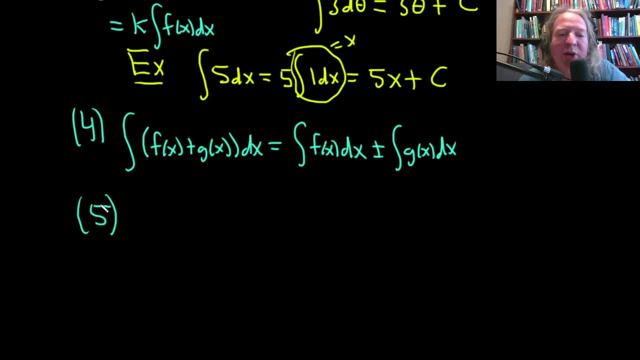 But basically it means you can integrate term by term. If you have five things, you can break it up into five integrals. That's okay as well. Five- This next one's really important. It's called the power rule. There's something about this. 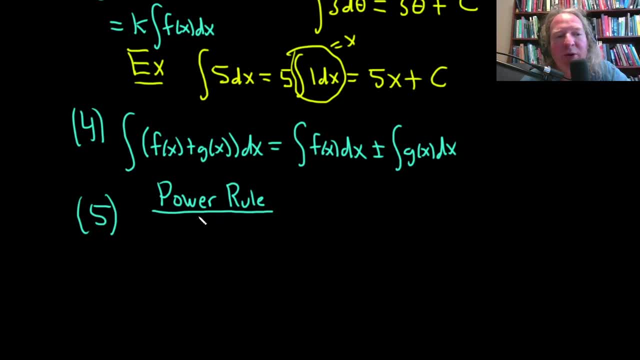 There's so many power rules in mathematics that it almost pains me to use the word, but it's okay, Context is key. So this is the power rule for integration. So if you have x to a power, say x to the n and you're integrating this with respect. 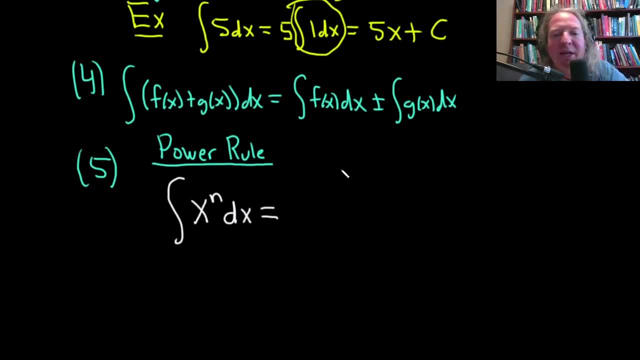 to x. so what you can do is basically you just take the exponent and you add one. So this is x to the n plus one, and then you just divide by the one and then you add your constant of integration capital C. 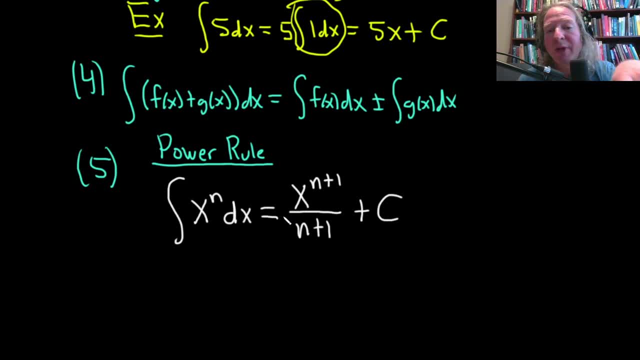 So very, very powerful rule. Now, if you're thinking like- I don't want to say a math person, but sometimes you get into the habit of thinking, hmm, when doesn't it work? Well, when doesn't this work? 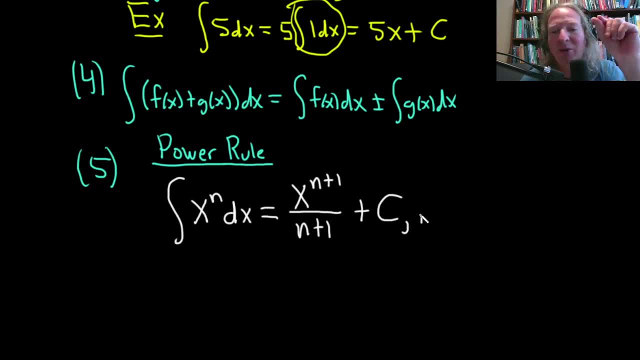 Well, if n is negative one, it doesn't work. So this is only valid for n not equal to negative one. Okay, And the natural question then to ask is: what do you do when n is negative one? I'll show you. 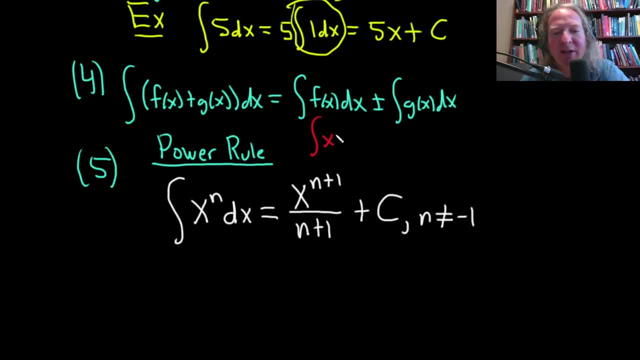 and i'm going to put it in red up here: if you have x to the negative 1, this is later. this is going to be the natural log of the absolute value of x plus c, and this, this is something you learn later in calculus. uh, we're not going to be discussing it in this video. it's taught much later. but for every. 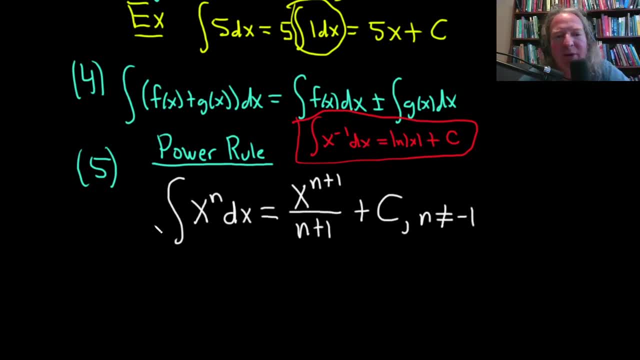 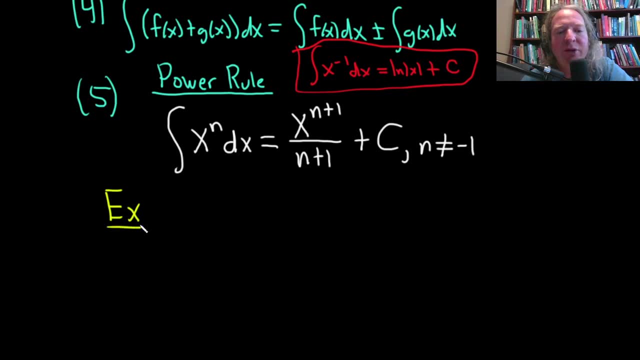 other choice of n? um. you can use this formula so very powerful. let's do an example right away, so you see it. so let's say we have to integrate x to the fourth with respect to x. so in this case a newcomer to the study of calculus might say: hmm, okay, so the exponent here is 4. this is the. 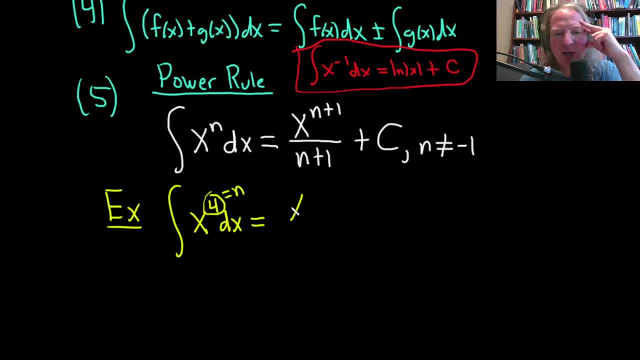 value of n. so if i'm going to apply this formula, it's x to the 4 plus 1 over 4 plus 1 plus c, and that would be 100, correct? and so this is equal to x to the 5 over 5. 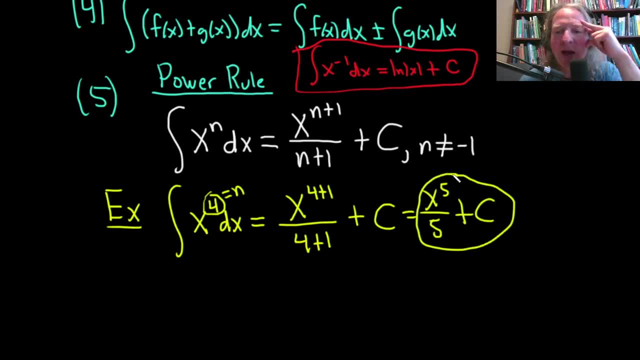 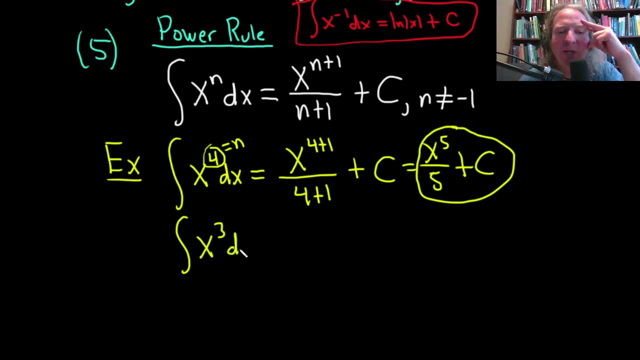 plus c. so this would be the answer now, in general, you do want to eventually move past this type of computation. you want to eventually skip this work because it really clutters your problem. so when you see a problem like this- let's just say x cubed x- you basically jump to the solution: 3 plus 1 is 4. 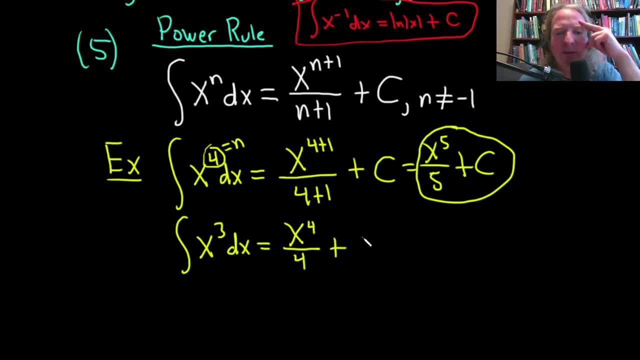 and then you just divide by the 4, like that, plus c. so you want to skip this middle step. it's not wrong, it's just it really like slows you down and it's just the math gets really long and involved. so anytime you can skip a step that's very, very easy to do mentally, like this it's. 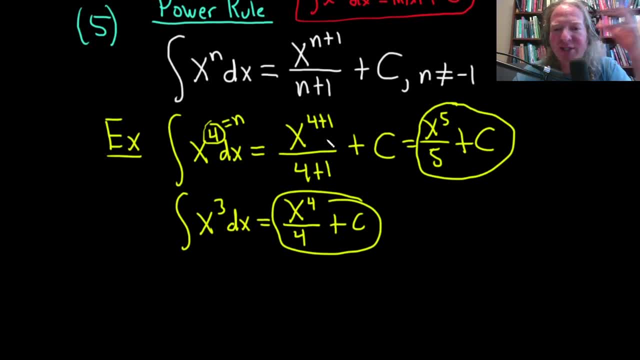 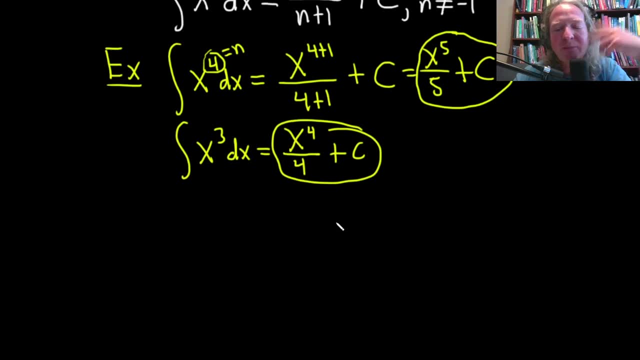 recommended that you do, and this just doesn't look pretty when you have six of these in the same problem, you know. so uh, worth just going to the answer. so very, very powerful formula. okay, i think what's left now are the trig functions. i guess i've been numbering these, so i'll call. 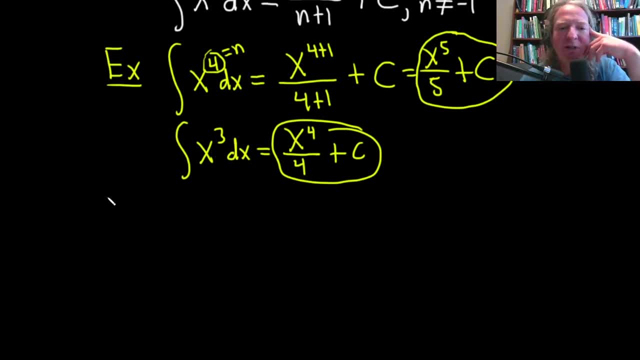 this one. six and the trig functions often intimidate people, because people see these formulas and they think, oh wow, i'm supposed to memorize all of these. you are, but at the same time you can think about them a little bit differently. so i'm going to show you how i 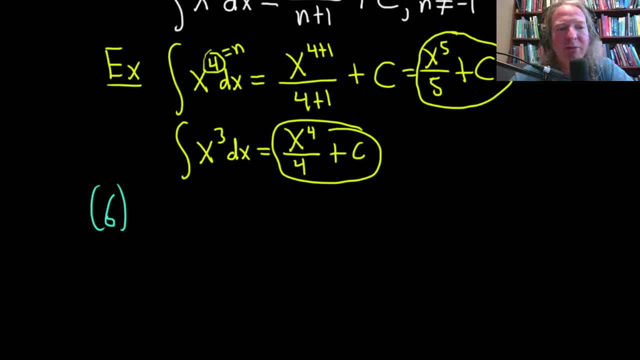 think about these and maybe that will work for you. so let me just switch colors here. for some reason, my pen got really thick. i had to. i can control how thick my writing is. watch this. i can write really thick, so i can write really thin. i'm just trying to find a happy ground here. here we go, let's try this one. 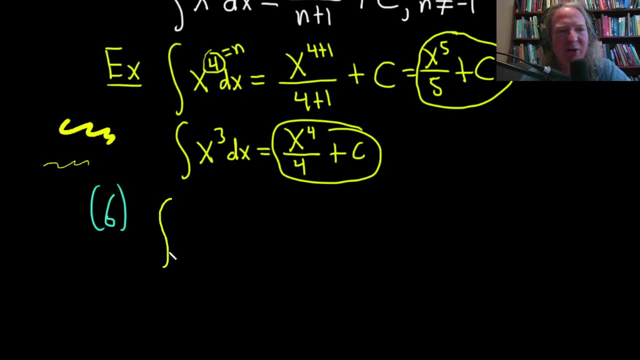 so let's try to integrate. that's pretty good. oh, i'm using graffiti pen. there we go. let's go back to pen. let's try cosine x. there we go back to regular writing, the integral of cosine x. so when you're trying to integrate cosine, you're asking yourself: what is a function whose derivative? 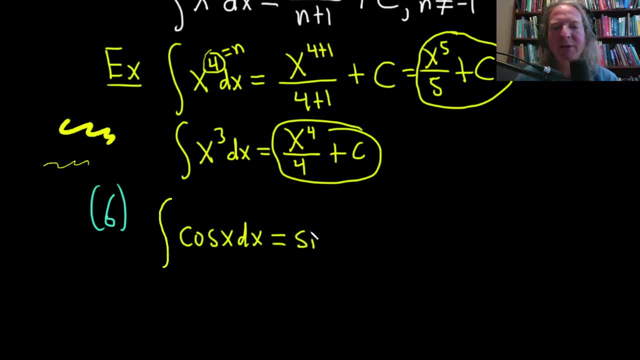 of cosine sine. this is sine x, but that's not it. we still need a plus c, so pretty easy. so whenever you look at the integral of cosine, if you don't have it memorized, you can memorize it. you can say, hey, the integral of cosine is sine, but maybe there's just those. you're just having a hard. 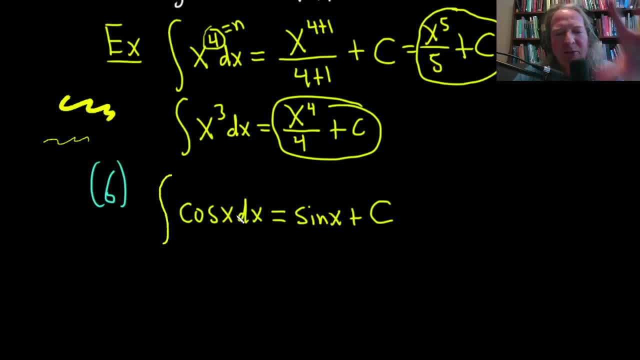 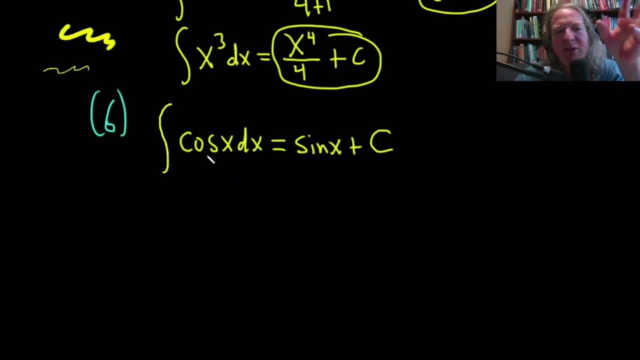 time finding room in your brain to memorize it, and you're just refusing to memorize things, which i have a habit of doing. i like to know how things are derived and it's just a habit. so you're getting cosine. you say i forgot what that was. oh, but wait, what's a function whose derivative is? 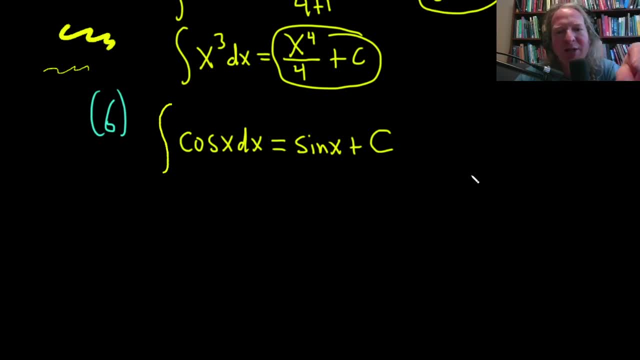 cosine, oh sine. the derivative of sine is cosine. yep, checks you differentiate this. you should get your integrand and it certainly works because the derivative of sine is cosine. what about this one? there's a reason: i did cosine first, because it's easier. this one's harder. 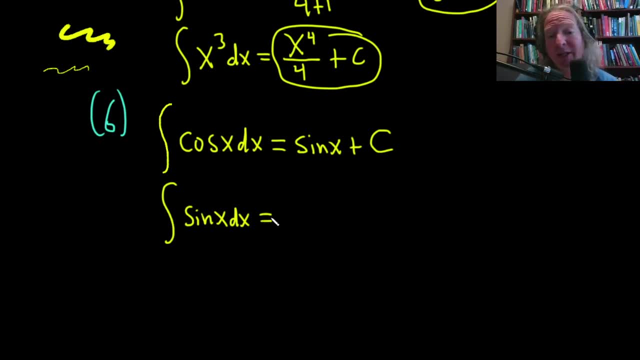 so what's a function whose derivative is going to be sine? well, the derivative of cosine is negative, so this is going to be negative, cosine x, and then plus our constant and you can check right. the derivative of cosine is negative, sine. we've already got a negative here, so negative and 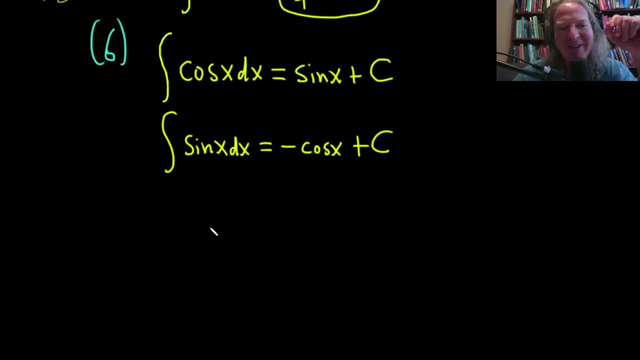 negative is positive, so life is good. how about this one here? secant x, tangent x. these are strategically picked, by the way, you might say: what about secant? why'd you jump to? secant, tangent, secant is a whole nother story. right, integration is not as easy as differentiation. the integral of 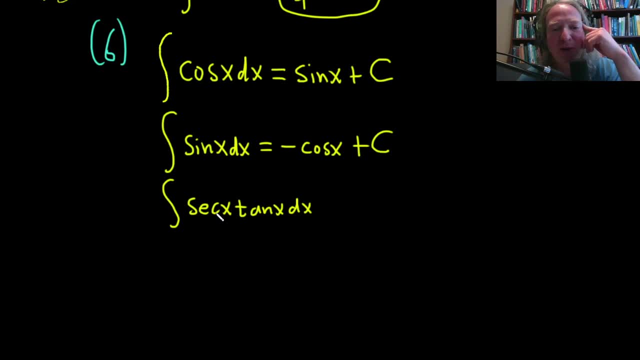 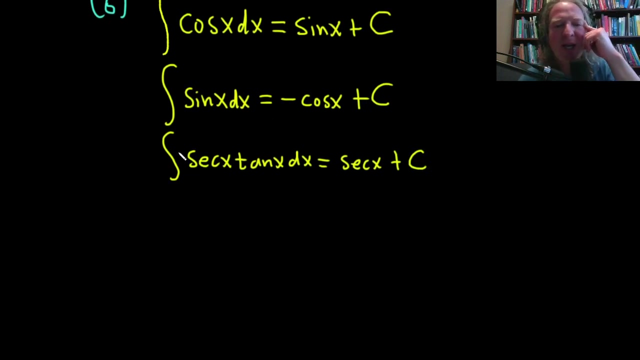 secant requires other techniques which we'll learn later. so you have secant times tangent. what's a function whose derivative is secant tangent? well, secant, this is the secant of x plus our constant of integration, capital c. and how about secant squared? that's another. 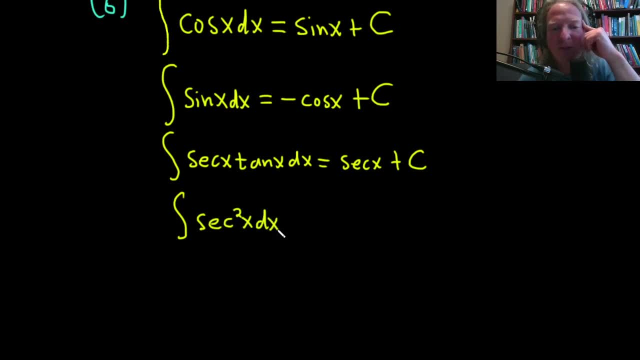 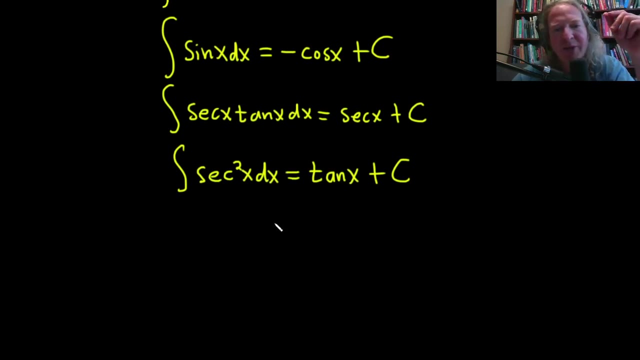 one we can do now secant squared: x, dx. so what's a function whose derivative is secant squared? well, we can set a derivative to take its Claro deriving term so that secant is even plus the derivative. this is to take the derivative square and the derivative of tangent is secant squared. 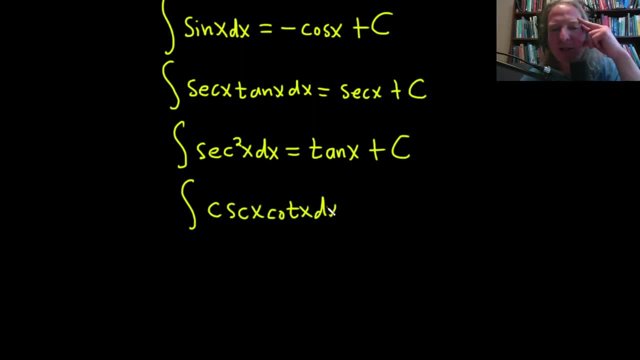 so we see that the derivative is just gonna be tangent x plus c. right, because the derivative of tangent is secant squared. and then we get to the unpopular ones, the ones that don't come up so much: cosecant x, cotangent x, dx. so what's a function whose derivative is cocca cotangent? well, the derivative of cosecant is negative cosete cotangent. so this requires a negative cosecant x plus c. 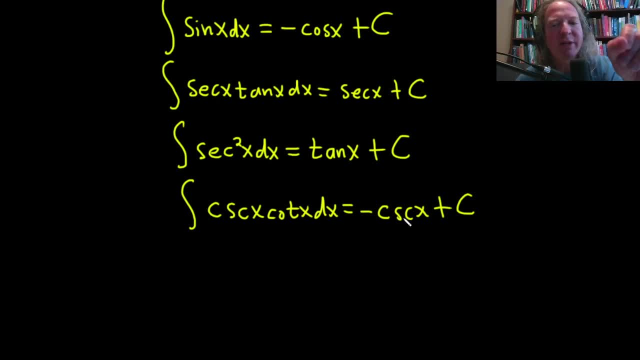 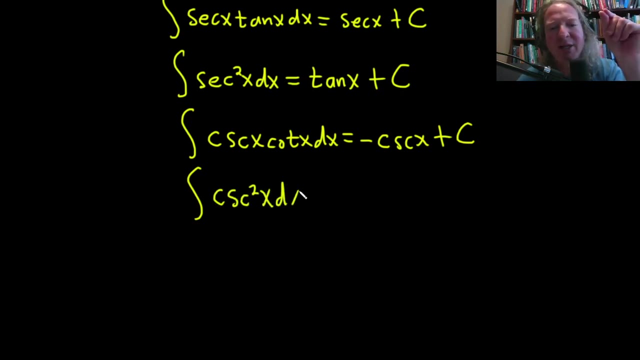 c. again, the derivative of cosecant is negative: cosecant cotangent. we've already got a negative, so it will become positive. and the last one we're going to discuss in this video, the last formula- i know it's a lot of formulas- is cosecant squared x, dx, and in this case you ask yourself what's a? 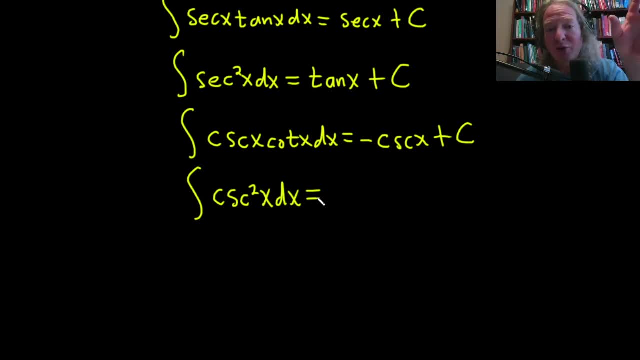 function whose derivative is cosecant squared. well, the derivative of cotangent is negative cosecant squared, so this is going to be negative cotangent of x plus our constant of integration, capital, c. so wow, that's a lot of formulas and usually when people first see this they're like: 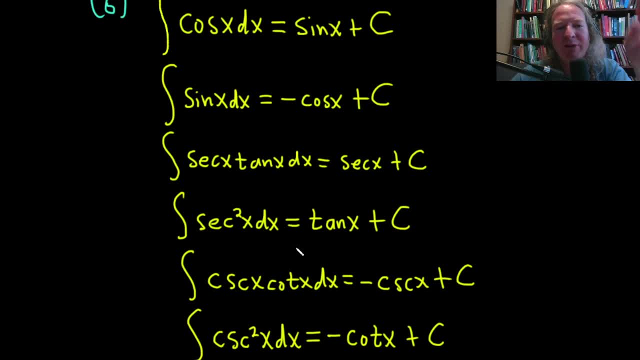 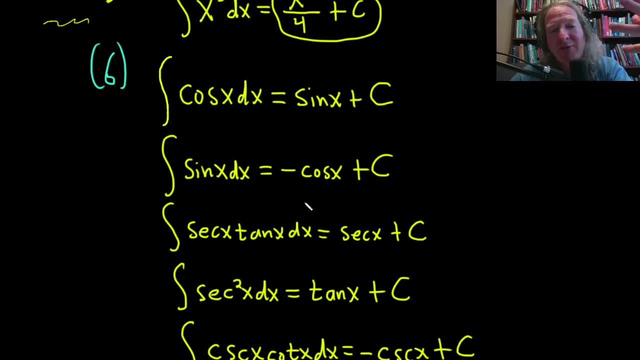 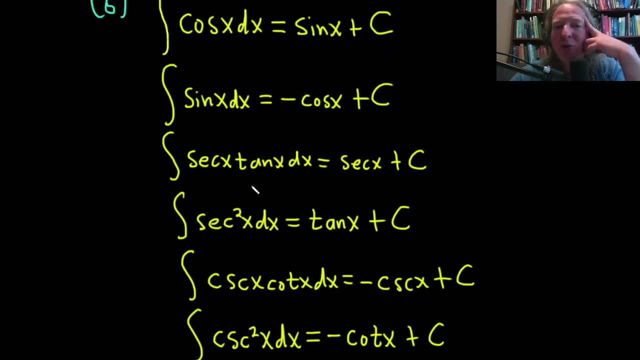 oh, mg, how am i ever going to know this? but how did i just go over it? right, it's just all derivatives, so it's really the derivatives that give you the integrals and at least for me, that seems to work better. it stays in my long-term memory. um, it just works better because you know you integrate other. 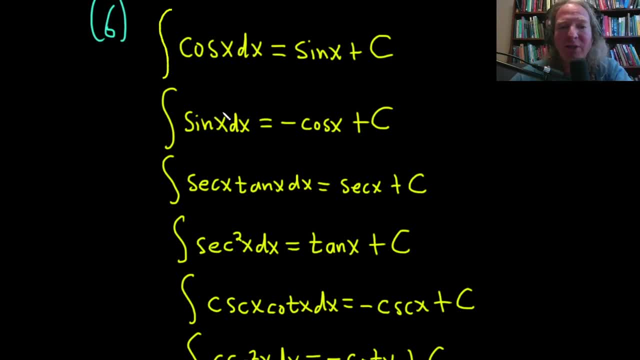 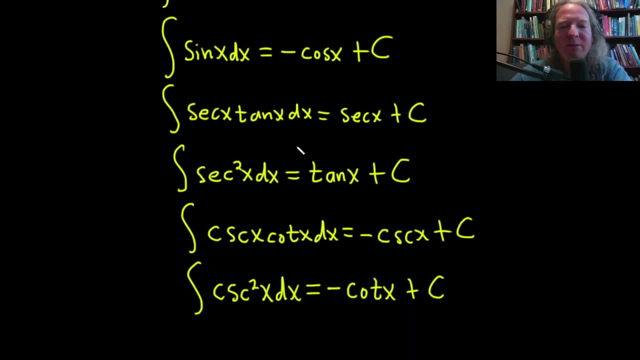 stuff besides these things you know you might have to integrate. you know you might have to integrate other stuff besides these things. you know you might have to sign the fourth power someday. that requires trig identities, requires a lot of knowledge. so, um, i just feel like the less you memorize, sometimes the better, and thinking about it in. 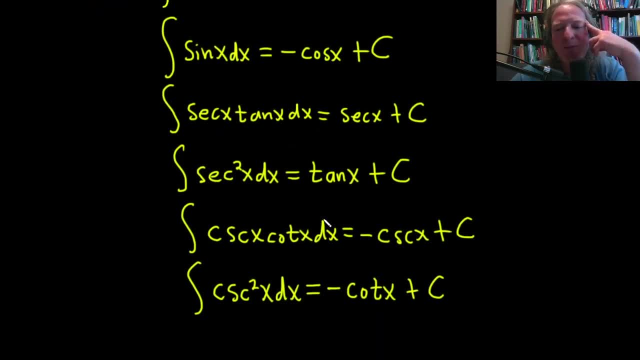 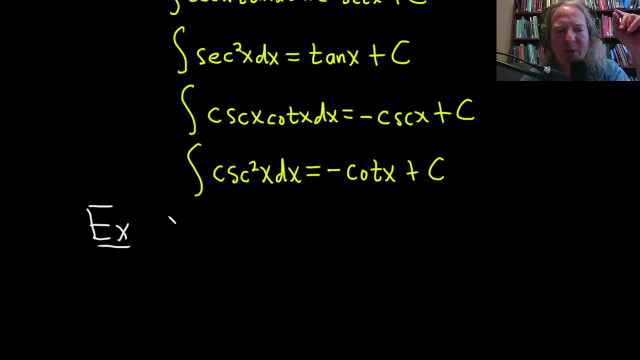 terms of differentiation. uh, makes it a little bit easier. let's go ahead and do an example. i'm going to switch back to white and let's just do a simple example here. let's say we have um x to the negative four- maybe not so simple- plus five plus.